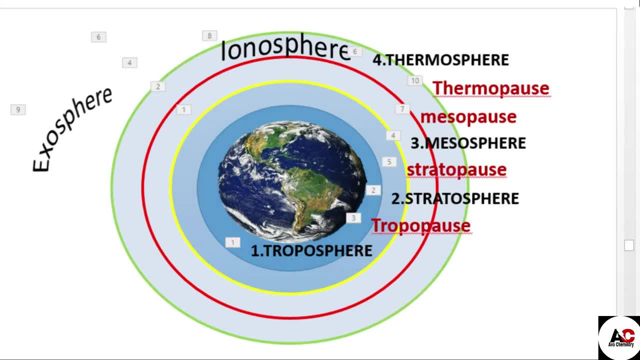 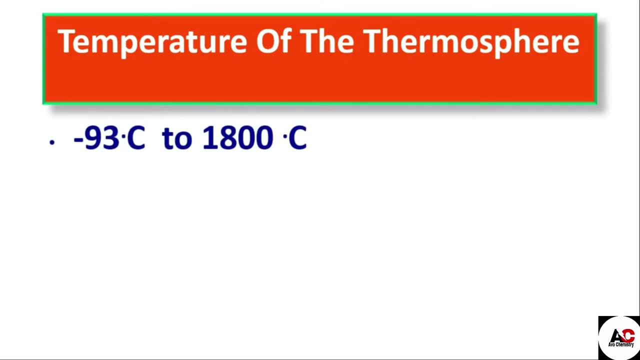 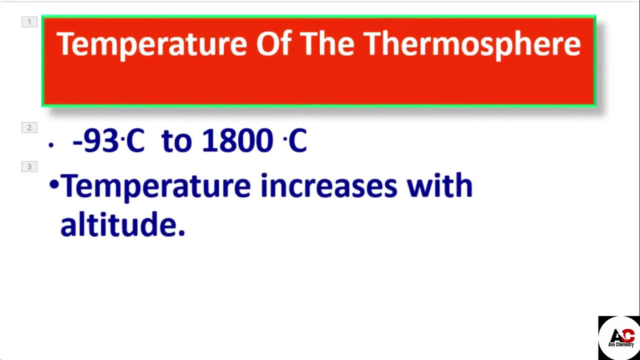 400 km to the 1000 km above Earth's surface is the exosphere Temperature of the Thermosphere – 93°C to 1800°C. That shows temperature increases with altitude. You can imagine how much hot this layer is At mesopause. that is the boundary between thermosphere and mesosphere, where temperature 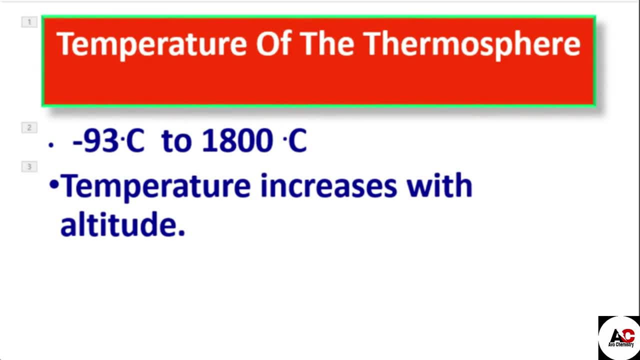 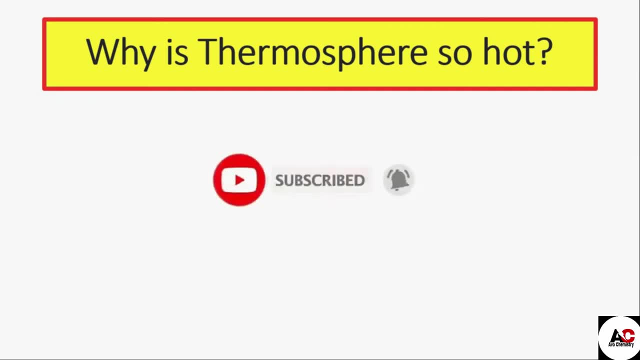 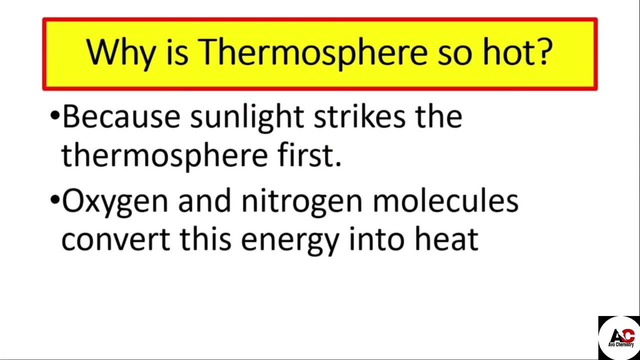 is minus 93°C. Its increases and reaches to 1800°C. But why is the thermosphere so hot? Because sunlight strikes the thermosphere first. Oxygen and nitrogen molecules convert this energy into heat. Yes, students, you know oxygen and nitrogen. 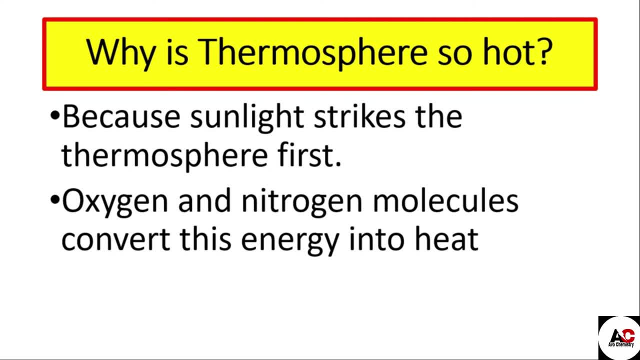 molecules are present in the thermosphere. These are the thermosphere's heat sources. These are the thermosphere's heat sources. Oxygen and nitrogen molecules convert this energy into heat. These molecules convert this solar energy into the heat energy. That's why thermosphere 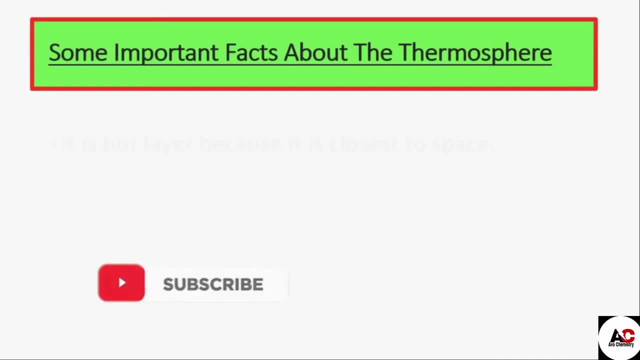 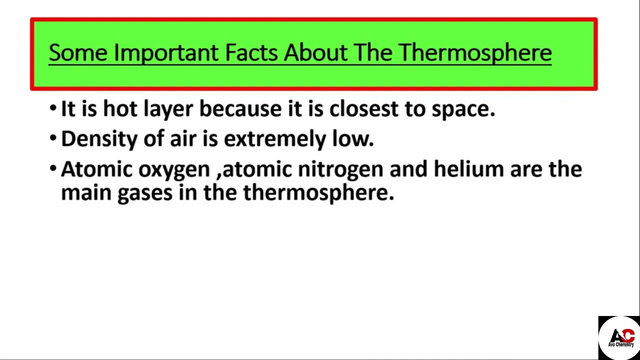 is so hot. Some important facts about the thermosphere. It is the hot layer because it is closest to the space. Density of air is extremely low. Atomic oxygen, atomic nitrogen and helium are the main gases in the thermosphere. Due to the very high temperature in the thermosphere, 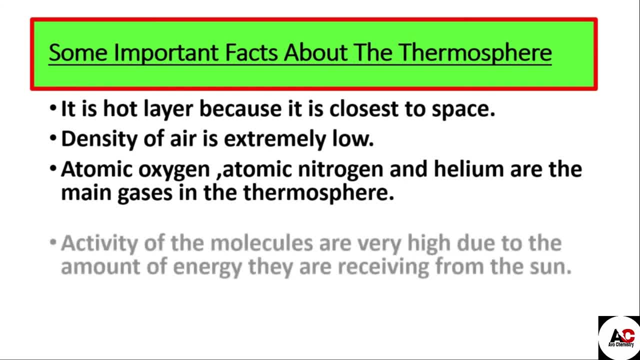 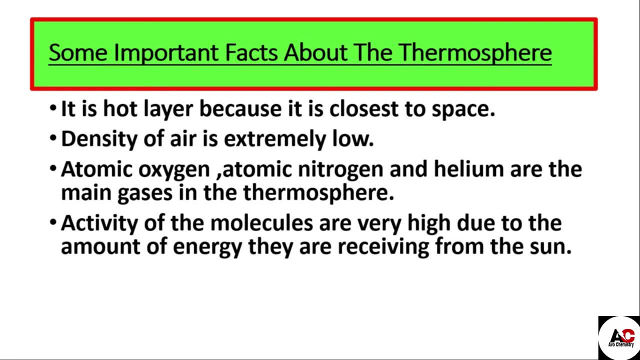 oxygen and nitrogen exist as their atomic forces. There's a bit of a Message behind this talk that they use this source of energy run man, and in this video I will give� you guys the reaction to cool thirteen or even break into colder lattice. So that's why this was the subject of unserplayed. 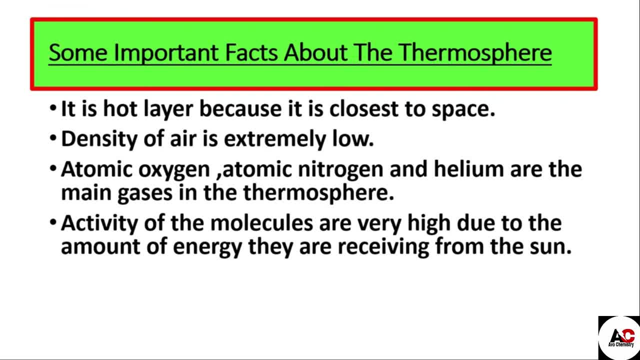 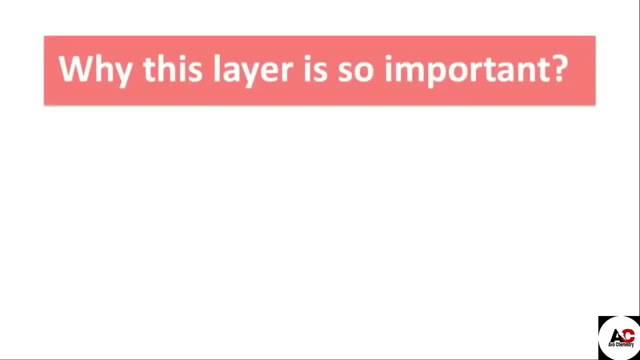 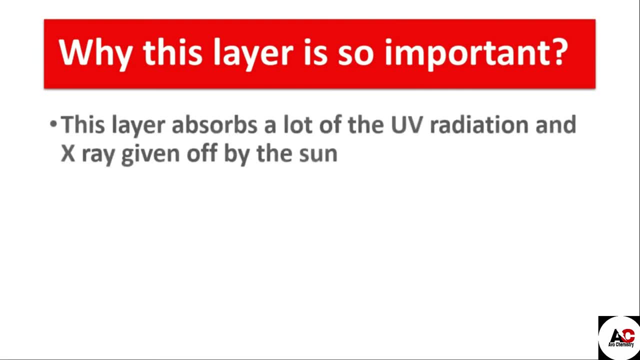 video. Wait a second, I want to tell you something important. convert their state into their atomic form. That's why Oxygen and Nitrogen exist as their atomic form, not in their molecular form. Why this layer is so important? Because this layer absorbs a lot of UV radiation and X-rays given off by the sun. That's why thermosphere.